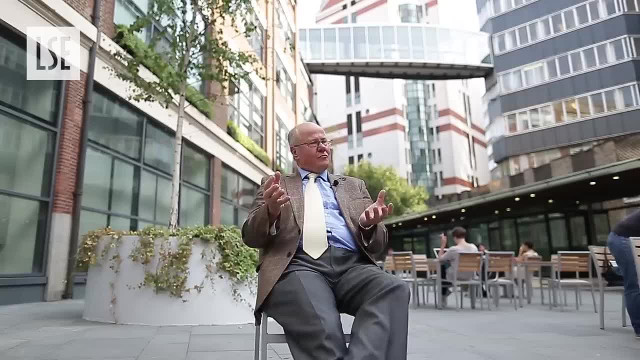 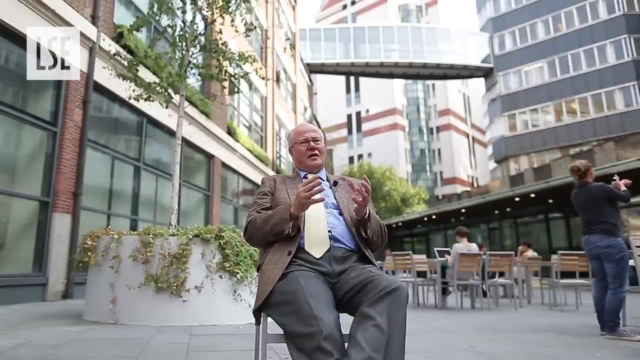 you can't build on at all because it's in the Greenbelt. So I've done several bits of research through the Spatial Economics Research Centre here at LSE, which was funded back in 2008 by BIS and the Department for Communities and Local Government, and we're still going strong. What we 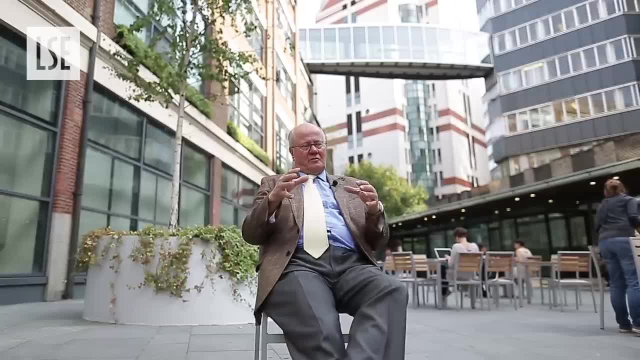 had within that was a lot of research. We've done a lot of research on how we can build more land over the years, on land, on land use planning. So we've had a set of research programmes relating to the use of land, relating to the economic effects of land use planning and relating to 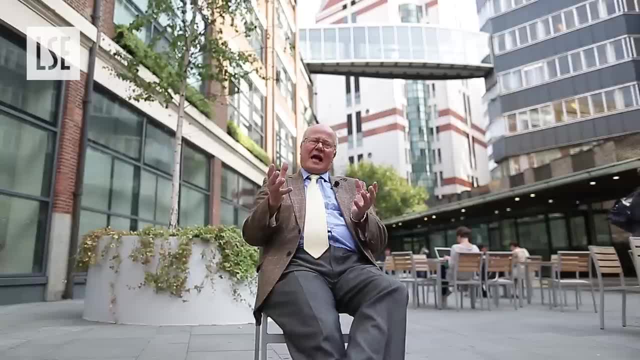 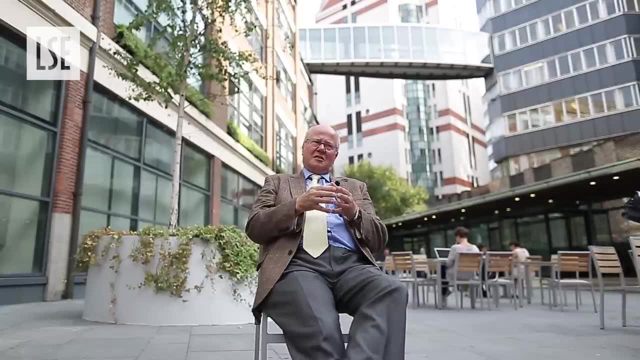 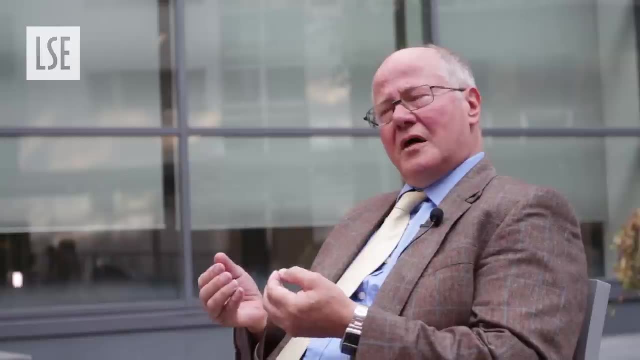 the housing crisis And we've published quite extensively out of that and it's had a lot of interest both in the particularly in government and in the political world, but also in the media. I have to say There's been a lot of media interest, mainly because people are really 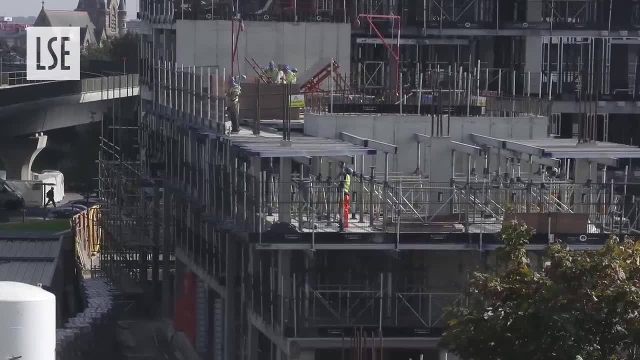 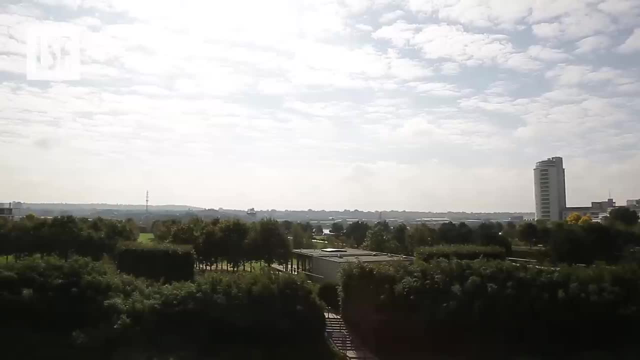 beginning to latch on to the fact that we have a lot of land. we have to be able to manage real housing crisis in England and it's self-inflicted. It's not something which we're sort of running out of land or whatever it may be. England is actually. 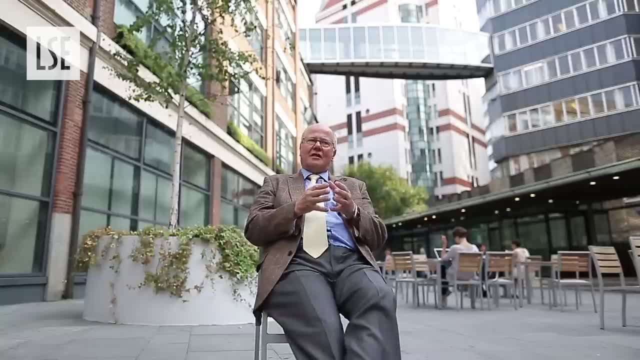 not much of it is built up. Only less than 10% of England is actually urbanised. People are sometimes not aware of that and it's because we have this complete limitation on land supply. It had an impact. First of all, I think it fed into 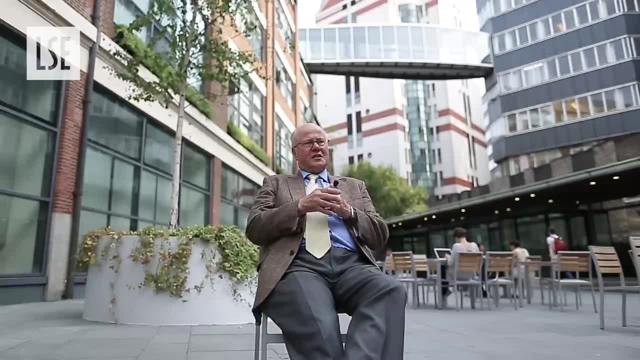 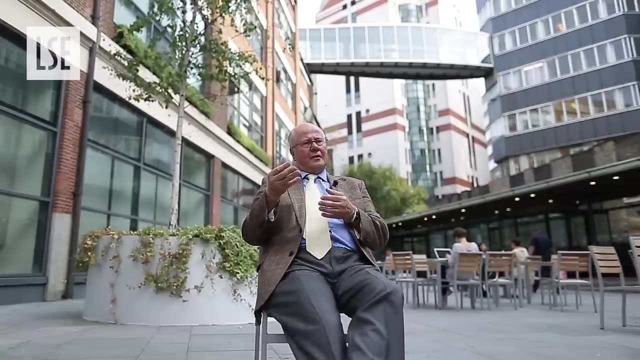 the Barker review. In 2003 the then government set up a strategic review of land-use planning system and its impact on the housing market called the Barker Review, and I was associated with that and quite a lot of our research began to feed into that review. and then they had a second review, which 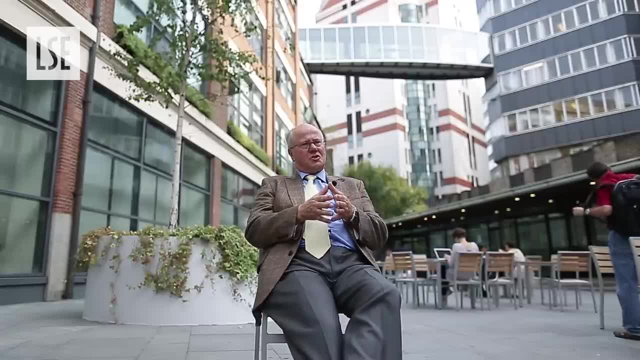 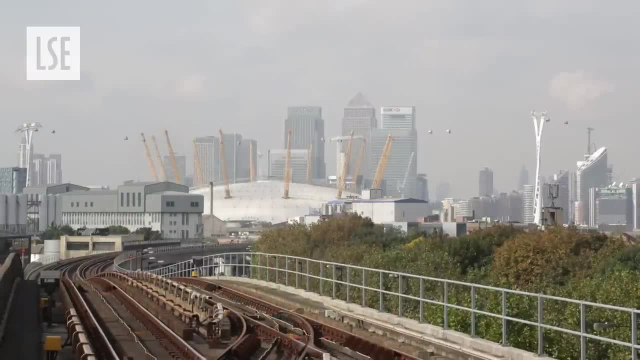 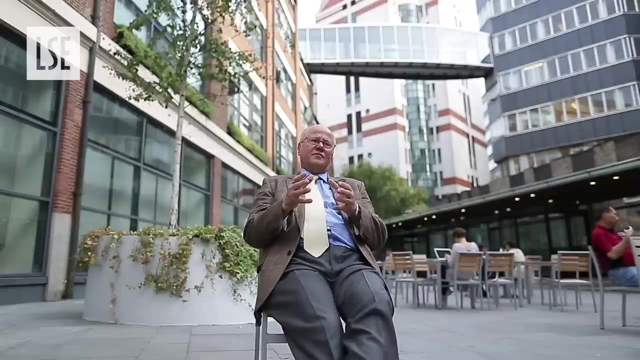 published in 2006 where they actually commissioned some research from us on the impacts of planning on the costs of offices. Very substantial. that turned out that in the highest, most restrictive parts of London there was something like an 18,000. hundred percent equivalent tax on the costs of constructing more office space. and so that that 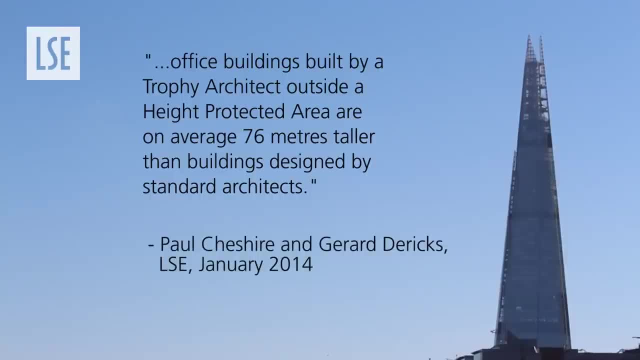 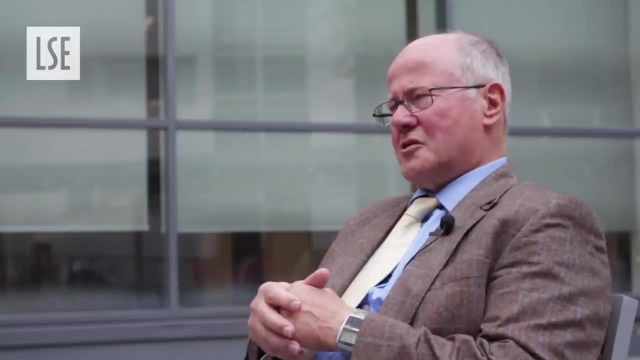 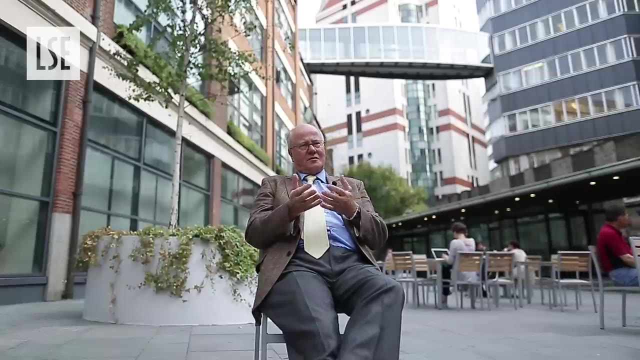 had a quite a significant impact, i think, on official thinking. it's led to the setting up of the reforms post barker, or it was influential in leading to those post barker reforms. that was swept away, of course. in 2010 we had a new government with new way, new ways of thinking. 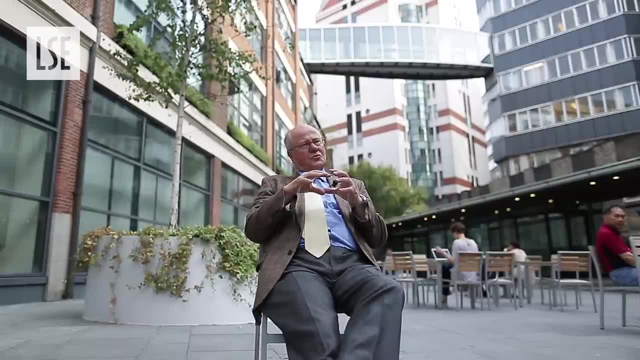 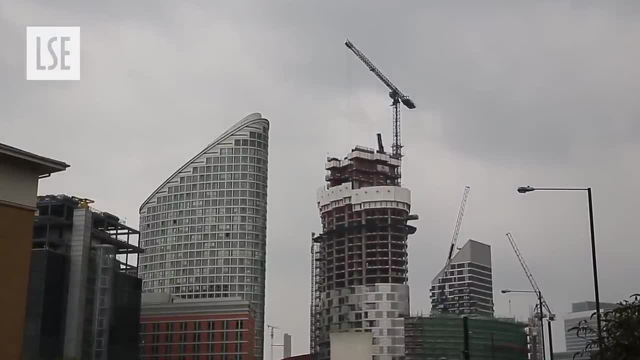 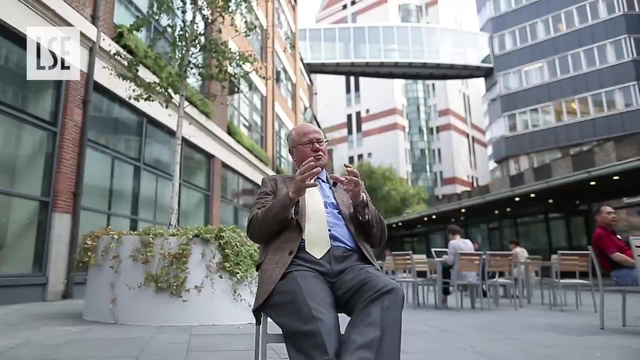 about it and they then to set out to first of all agree to this community infrastructure levy. the idea is to have an impact fee on the uplift in land values which is created by giving planning permission, but the uplift attacks, which relates to the costs that that development imposes on. 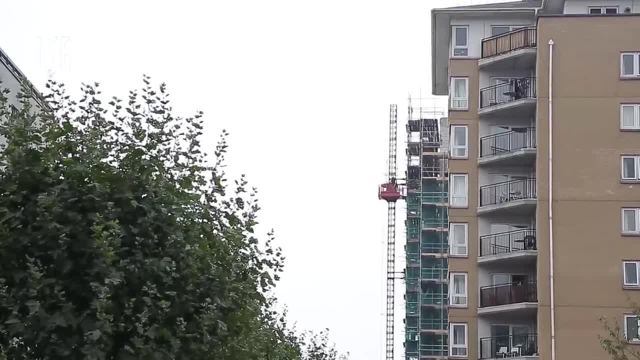 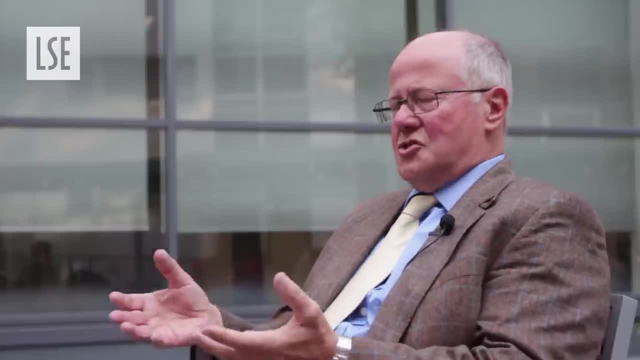 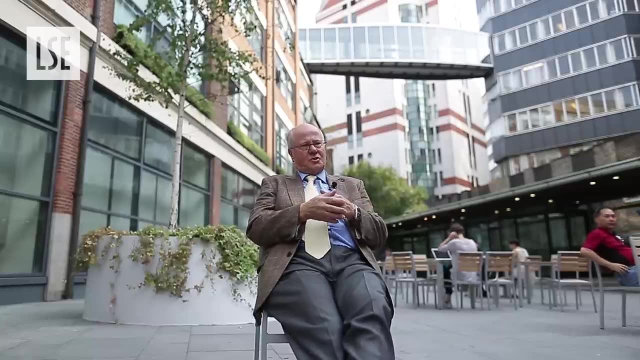 the community because, of course, if you build more houses, this does have a cost on local people. uh, becomes more crowded, more congested, infrastructure gets, gets overused, there's noise and disruption. people lose their views. so you do need to have compensation in order to offset for those costs And the community infrastructure levy. 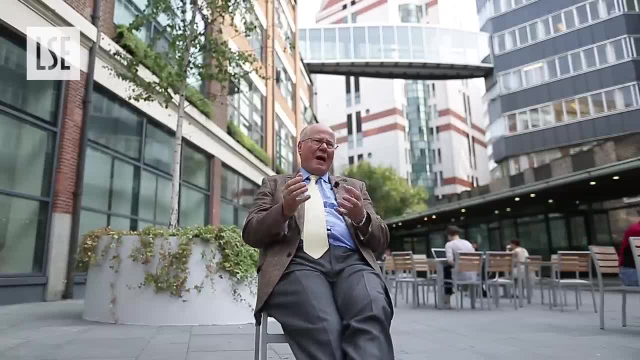 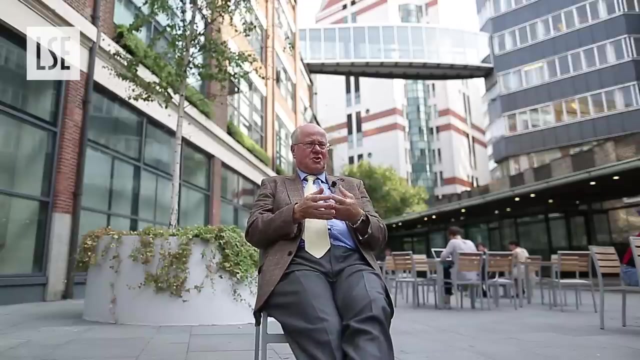 was an attempt to do that more transparently than the existing system did. Secondly, the government set out to try and entirely reform and recast and simplify the basic planning policies in this new national planning policy framework document, which did take on the basic message that we had been trying to communicate, which is that development is not necessarily 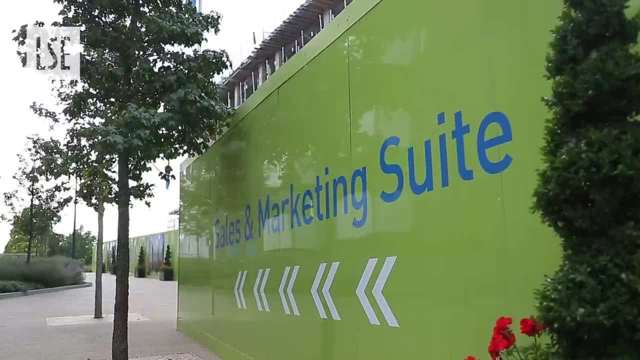 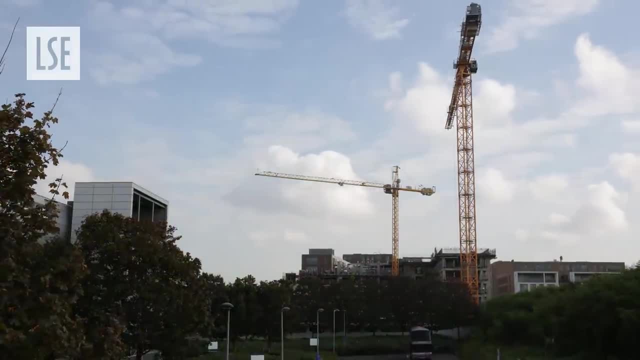 bad for the environment. What you need to do is protect environmentally valuable land and high amenity land and open spaces, whereas it doesn't take very much land to build on. So if you've got development which is sustainable, then there should be a 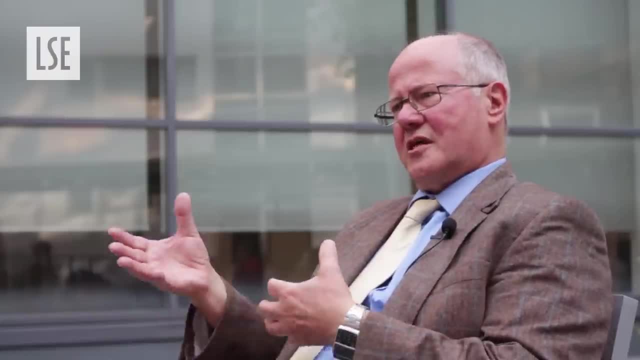 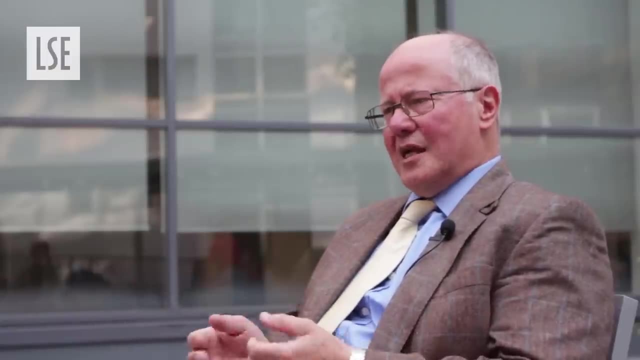 presumption that it's okay. The problem is, of course, if it's going to be destroying important habitats or environmental land or taking up land which is valuable for recreation or amenity, And one of the elements in that was to recognise that you had to take account. 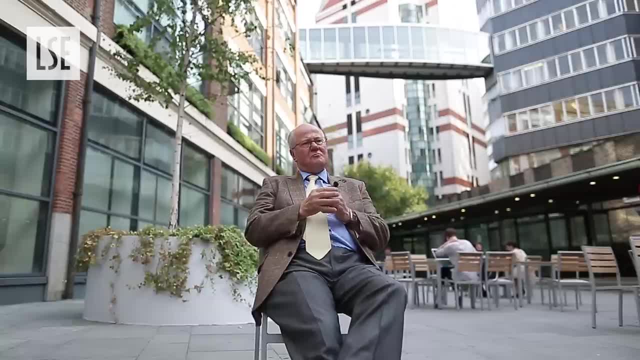 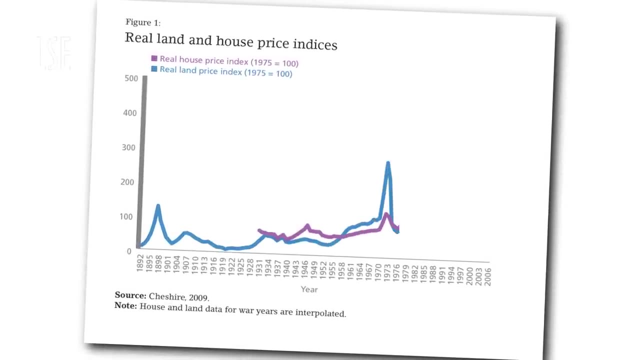 of the impact on prices, because being so restrictive on land supply, which our policy has been over the last 50, more than 50 years since 1955, means that if you're going to get permission to convert an acre or a hectare of agricultural land on the edge of London, 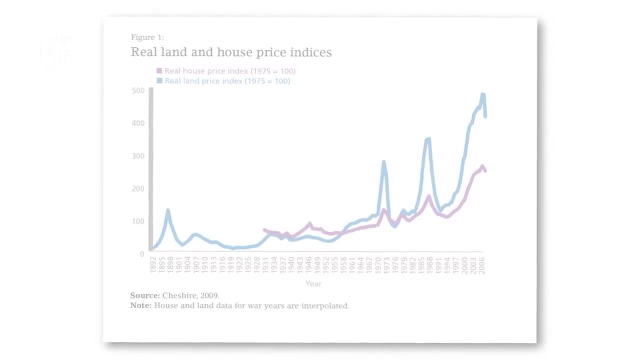 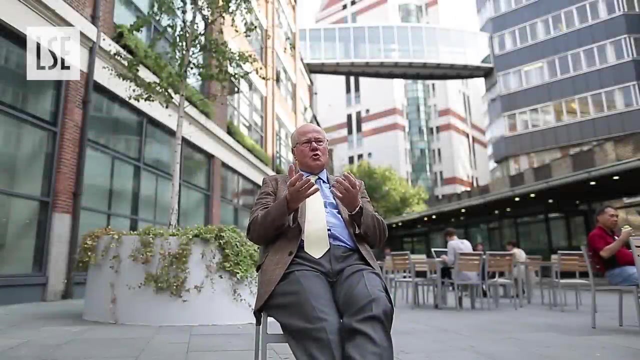 from agricultural land into housing, then the value of it goes up from sort of £10,000 to £20,000 a hectare to perhaps £10 million a hectare. So there's a huge price distortion in the land market which is reflected in what we have to pay for housing. So the argument: